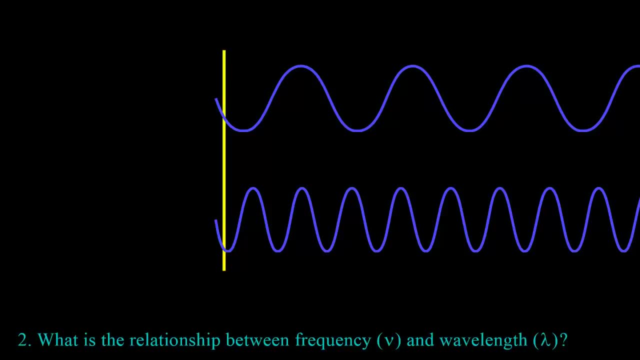 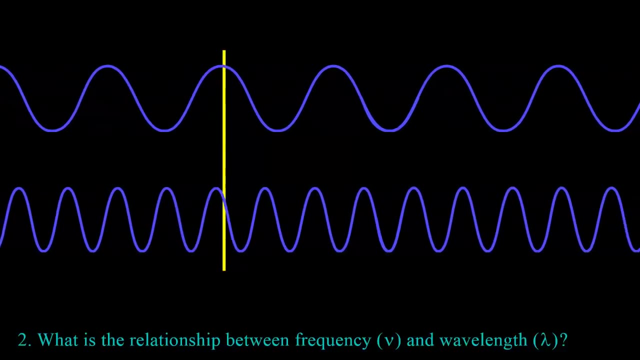 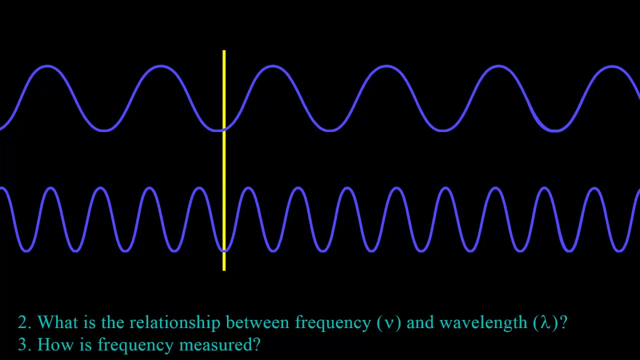 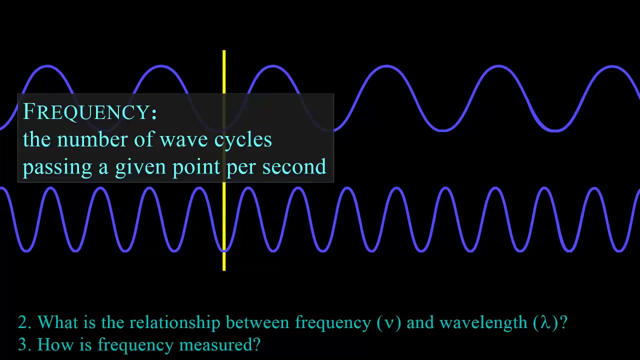 To bring the point home, each wave will flash as it passes the yellow line. You can see that the shorter wavelength flashes more frequently than the longer wavelength. But before we connect this with light waves, we need to understand how frequency is measured. Frequency is defined as the number of cycles passing a given point per second. Here we 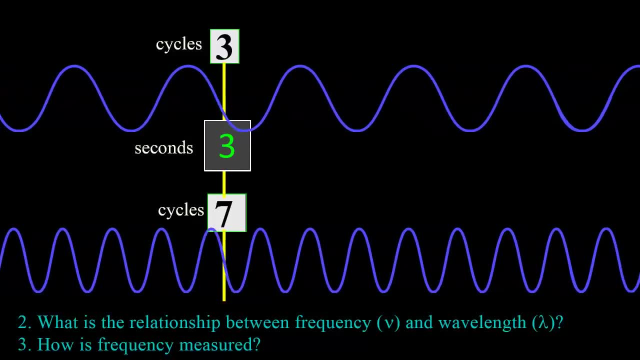 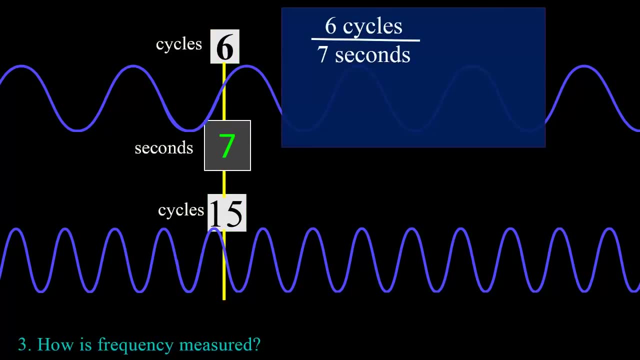 put a counter on both the wave cycles and on time For the top wave, we see that six cycles passes through in seven seconds. Dividing six cycles by seven seconds gives a frequency or nu of 0.86 cycles per second. The shorter wavelength at the bottom gives a frequency 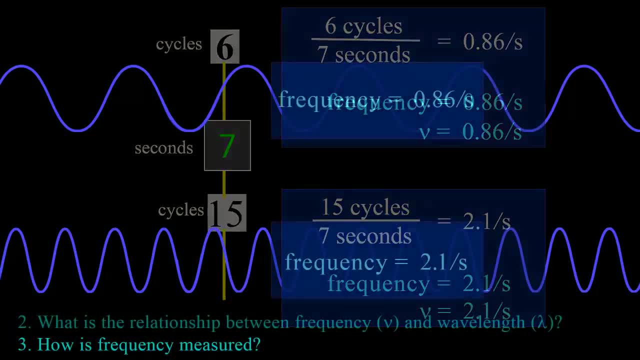 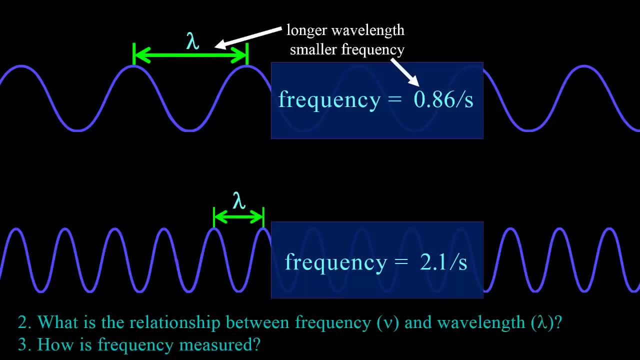 of 2.1 cycles per second. So here we get a better view of the relationship between frequency and wavelength. The longer the wavelength, the smaller the frequency, and a shorter wavelength has a larger frequency. So frequency and wavelength have an inverse relationship. 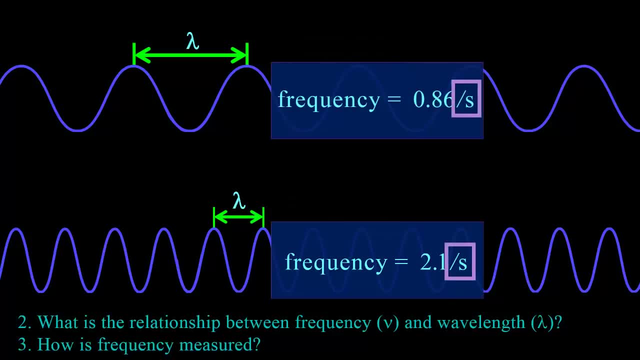 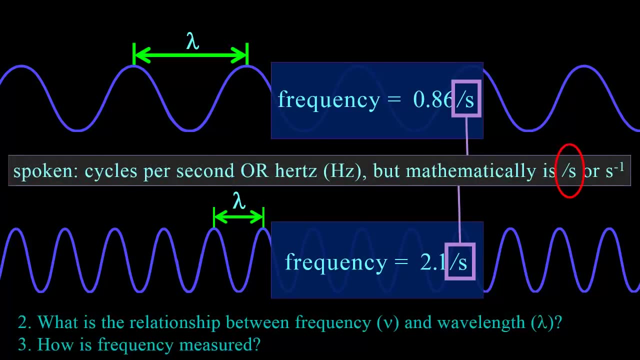 It is important to notice here that the unit for frequency is simply per second. We say cycles per second, but mathematically it is only expressed as per second, which is often expressed as s to the negative one. Finally, hertz is another way to express cycles per. 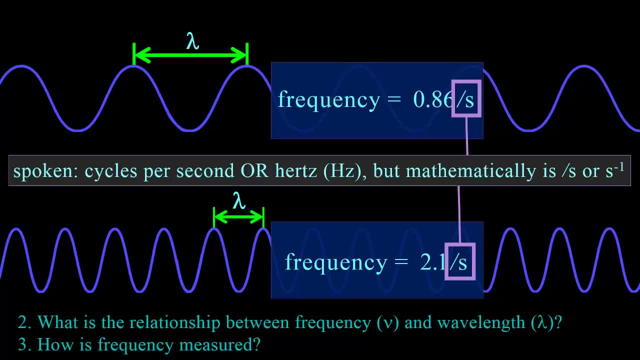 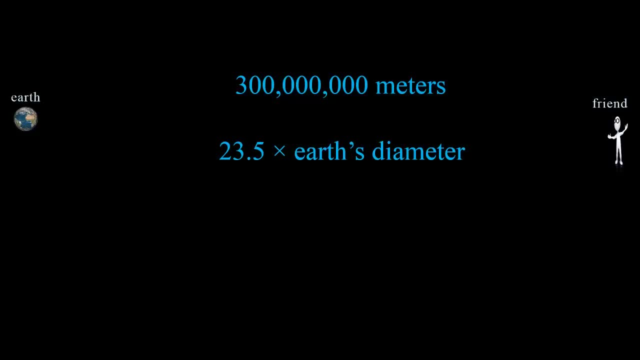 second, All of these are in common use. Now let's talk about the speed of light, so we can tie it to frequency and wavelength. Speed is how long it takes to get from one place to another. Let's say you happen to have a friend standing 300 million meters away from Earth, or about 23 and a half times. 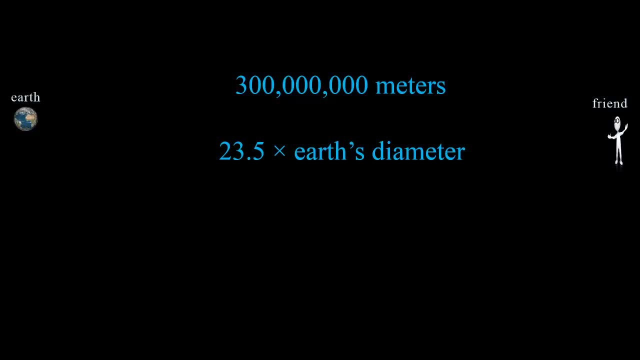 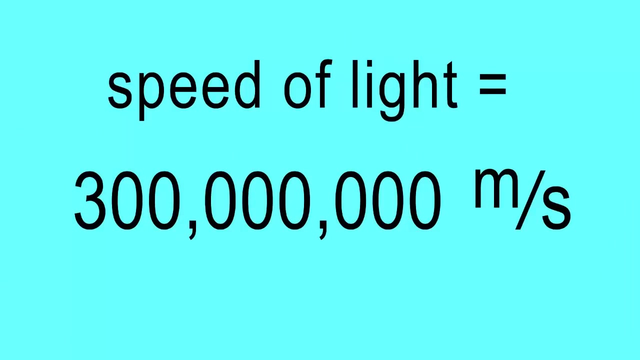 the Earth's diameter, waiting with great anticipation for a signal from you standing on Earth. How long would it take your friend to see a single wave of light emitted from your red laser? Well, the speed of light happens to be 300 million meters per second, And so it takes. 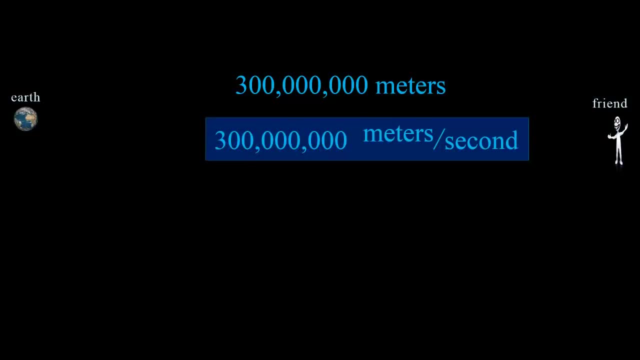 one second for the flash of red light to reach your friend. Interestingly, when your friend sees the light, they actually are seeing what you did one second in the past. Let's look at something slightly more realistic: the Moon. It would take 1.23 seconds for your. light to go 370 million meters to the Moon. The sunlight we see to increase the speed of light is only 0.03 charged. мамetern per reflected from the moon's surface takes 1.23 seconds to reach the Earth. 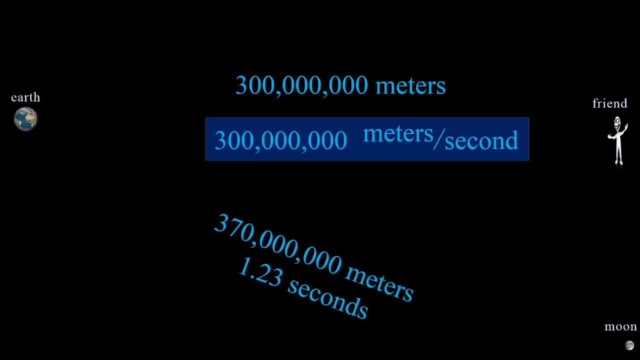 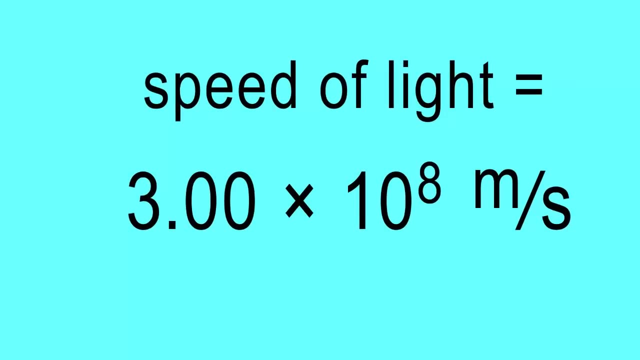 And so when we look at the moon, we see what happened on the moon's surface 1.23 seconds in the past. The speed of light is normally given in scientific notation 3 times 10 to the 8th meters per second. 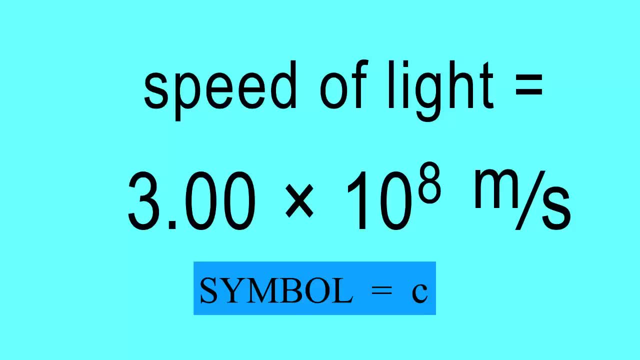 And, yes, it has its own symbol, which is the lower case c, so c. the speed of light is 3 times 10 to the 8th meters per second, 300 million meters per second. Knowing that the speed of light is a constant will give us access to the mathematical relationship. 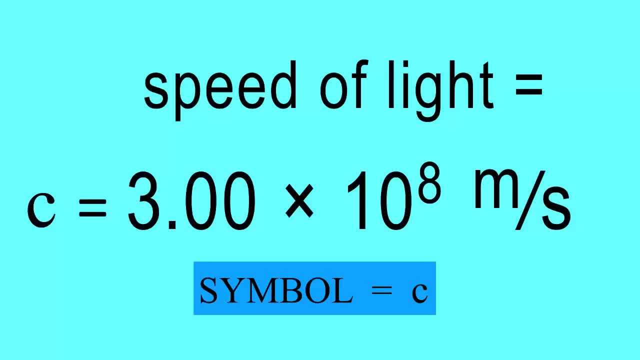 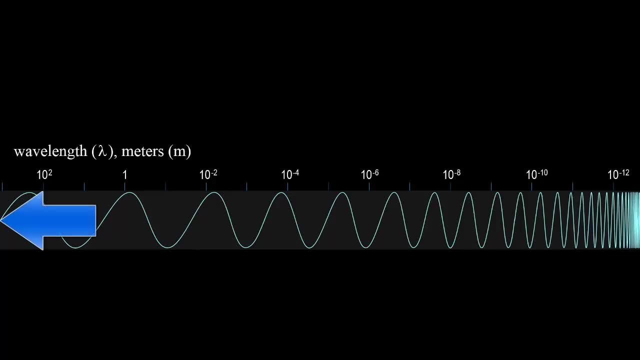 it has with wavelength and frequency. Let's derive that relationship. First. you should know that the wavelengths of light cover a very wide spectrum from greater than 100 meters to less than a trillionth of a meter. A narrow band within that range are light waves that we have evolved to detect with. 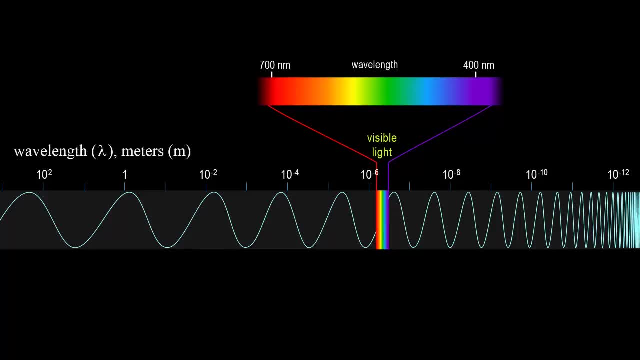 our own nervous system, And so this is the visible spectrum. With wavelengths of light, we have a wide spectrum. It's between 400 and 700 nanometers, with each color corresponding to a different wavelength. Other wavelengths correspond to a variety of different waves, such as radio waves, microwaves. 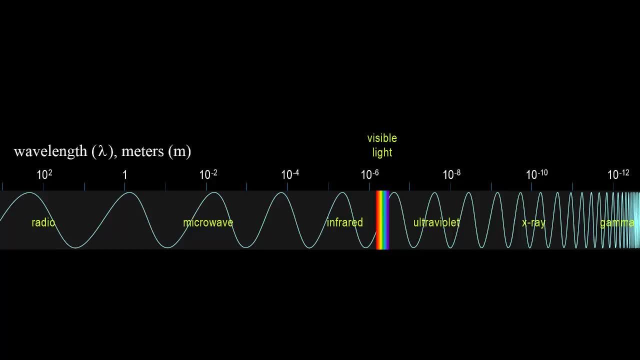 infrared, ultraviolet x-rays and gamma rays. These are simply names given to different ranges of wavelengths. However, it is important to remember that all are moving at the same speed: 3 times 10 to the 8th meters per second the speed of light. 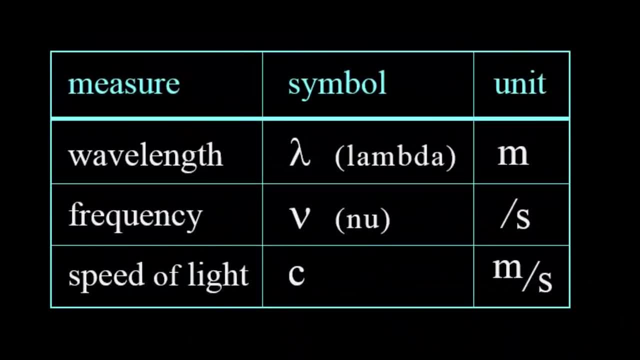 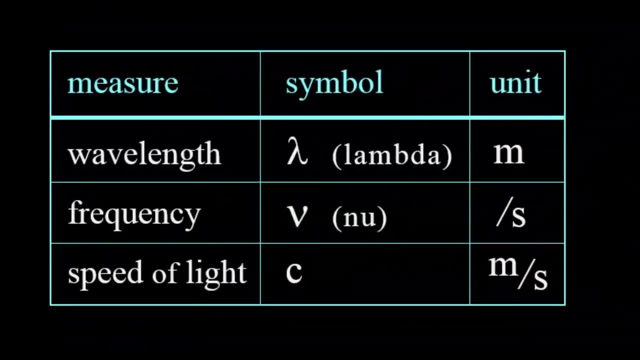 Before we head into the final lap, let's make sure we have our symbols and units straight, which can often be confusing. Each symbol simply represents a specific measure. It is really the unit that is most important. The unit gives meaning to the number of the measurement. 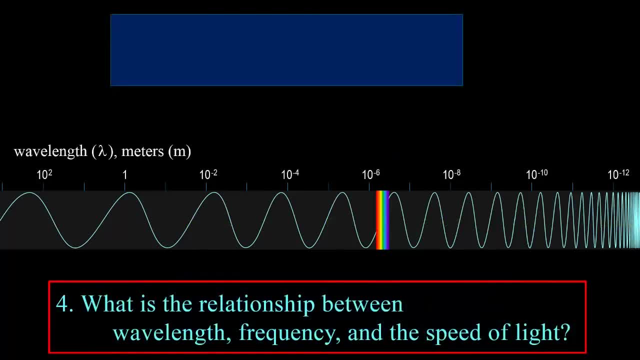 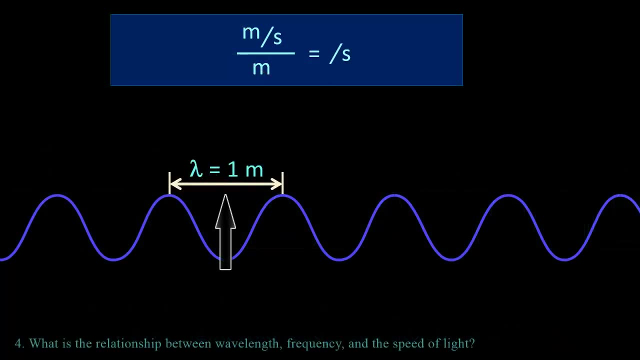 So how are wavelength and frequency related to the speed of light? If we look at the units of speed and wavelength, we can see that dividing meters per second by meters will cancel meters And we get per second the unit of frequency. Let's say we have light with a wavelength of 1 meter. 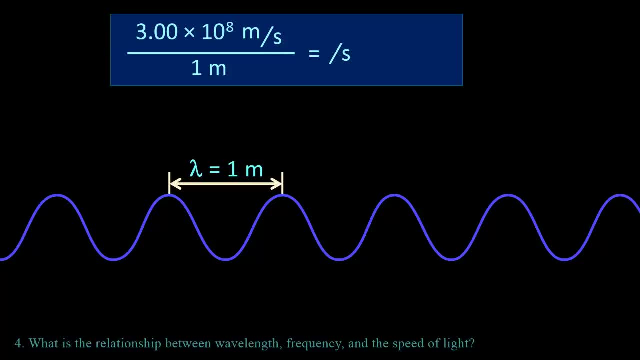 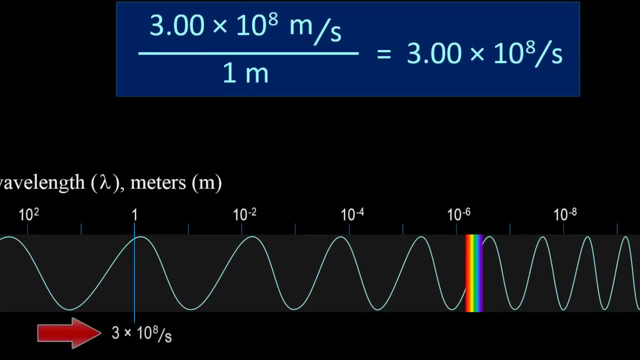 Its speed is 3 times 10 to the 8th meters per second, And the division gives us a frequency of 3 times 10 to the 8th cycles per second. So a wavelength of 1 meter corresponds to a frequency of 3 times 10 to the 8th cycles. 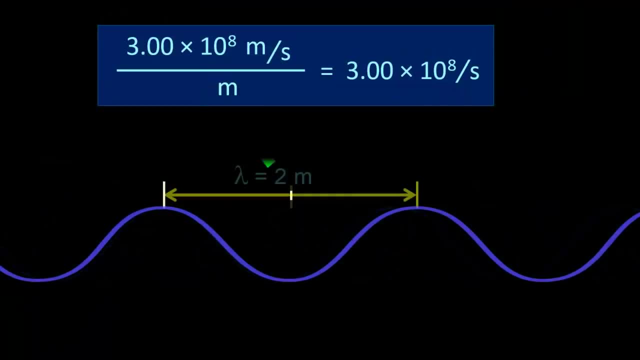 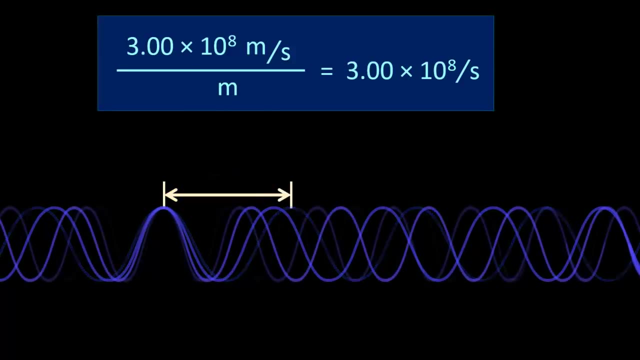 per second. If we have a wavelength of 2 meters, we get a frequency of 1.5 times 10 to the 8th cycles per second, And if we have a wavelength of 0.5 meters, we get a frequency of 6 times 10 to the 8th. 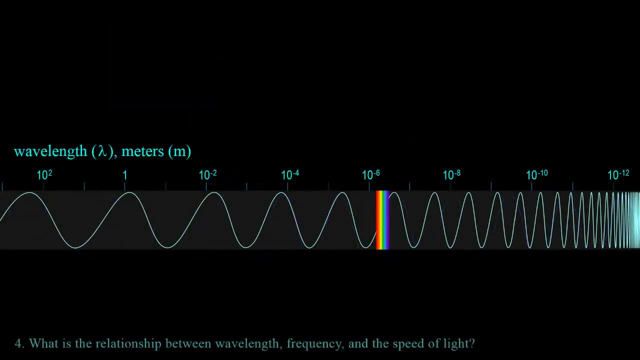 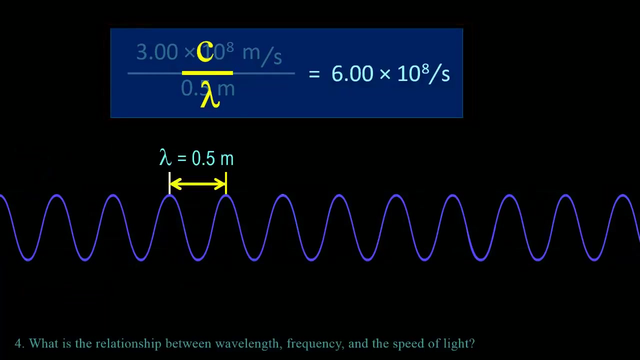 cycles per second. So any wavelength has a corresponding frequency, as we can see here. Now we can start putting it all together using symbols to arrive at our equation relating wavelength, frequency and the speed of light. So the speed of light divided by wavelength equals frequency. 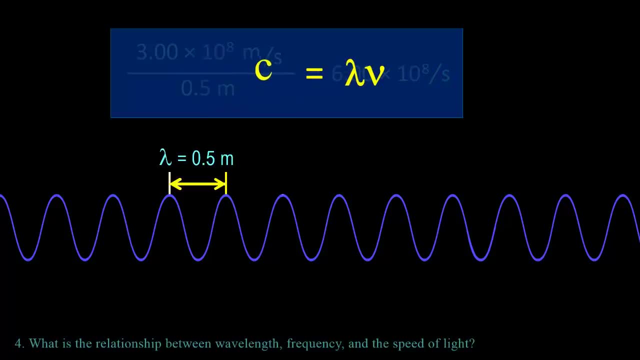 We can start putting it all together using symbols to arrive at our equation relating wavelength. We can algebraically rearrange to C equals lambda nu, but it is generally represented as lambda nu equals C, so we will keep that. If we rearrange our original calculation to lambda nu equals C, we can see that the units 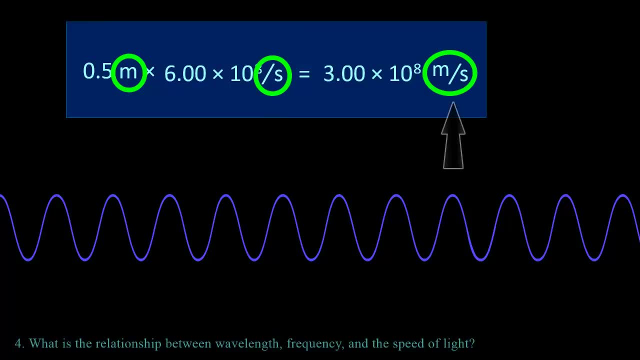 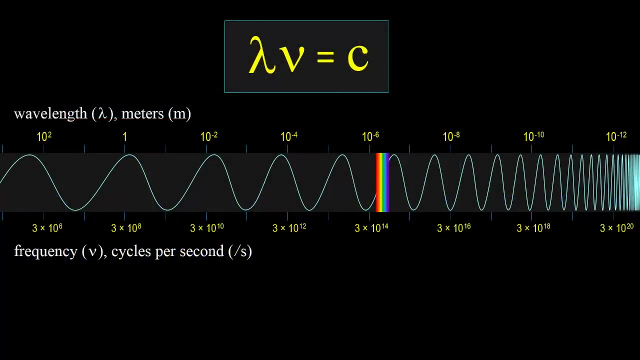 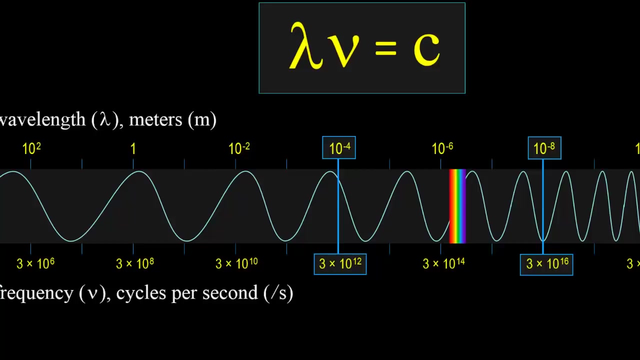 work out correctly: Meters times per second equals meters per second. So lambda wavelength times nu. frequency equals C- the speed of light, And therefore each wavelength has a corresponding frequency And any wavelength multiplied by its corresponding frequency will always give the speed of light. 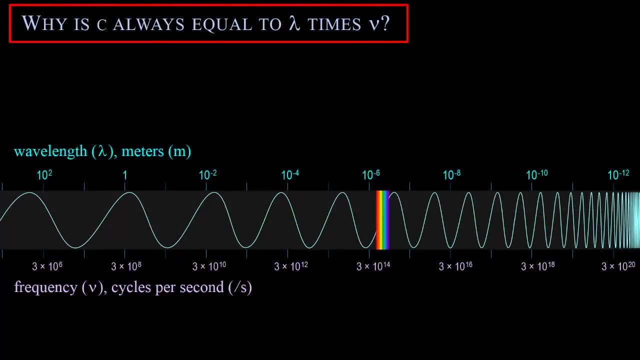 You should now be able to answer our last question: Why is the speed of light always equal to wavelength times frequency? Well, I hope you noticed in this illustration that wavelength decreases going toward the right, Frequency increases going toward the right. What you should also notice is that this inverse relationship is an exact proportion. 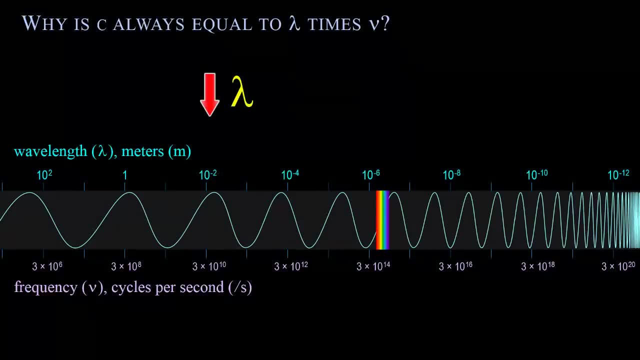 Because the speed of light is constant, any decrease in wavelength is accompanied by a proportionate increase in frequency. It is a simple relationship shown by the equation itself. but the equation comes out of the nature of light. a simple example of the beauty of mathematics giving a description of a natural 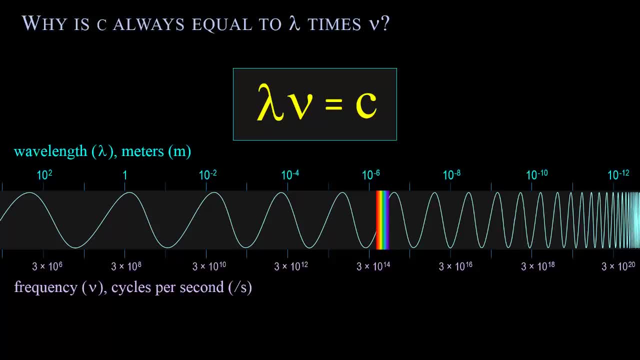 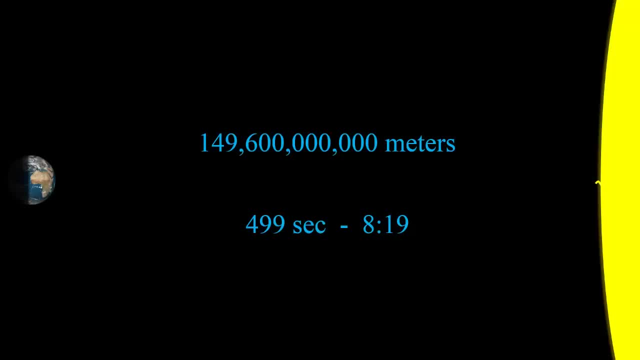 phenomenon: The relationship of frequency, wavelength and the speed of light. So that should be the end of the video, but I have another illustration to show you. I originally was going to show the speed of light by showing a light wave traveling from.